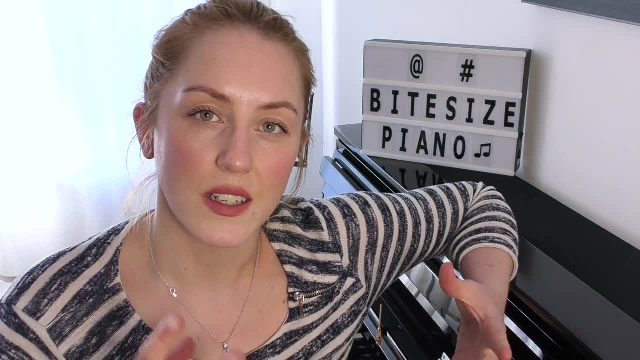 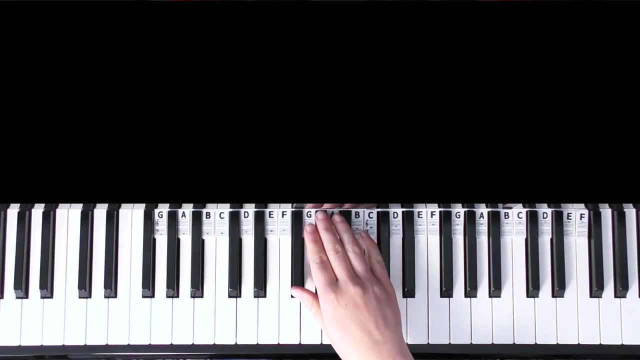 of how to make your accompaniment sound slightly more interesting rhythmically. So let's go to the piano and I will show you the first pattern. So the first one is going to be the most simple one. So we're going to use the same chord progression, which is just a four chord. 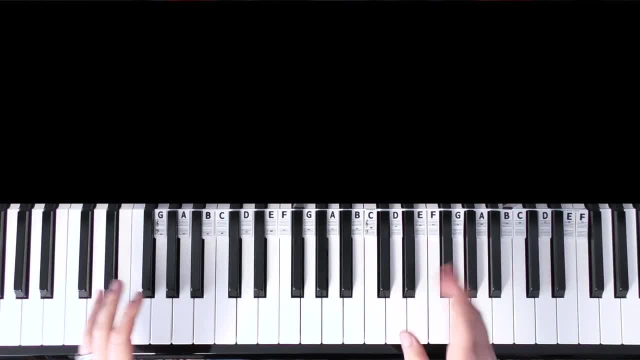 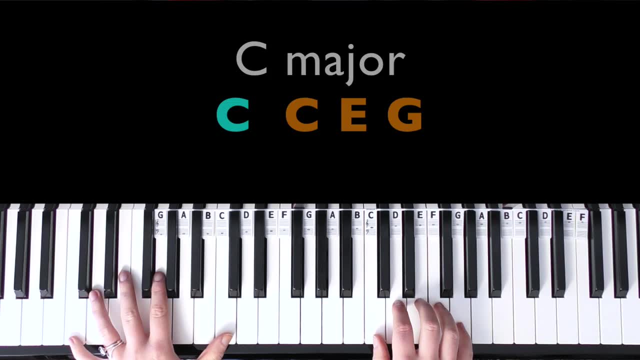 chord progression. So I'll teach you the chords first if you want to play along. but again, this is just to give you ideas of how you could play a chord progression if you're unsure. So we've got C major, So it's C's in the left hand, C, E, G. 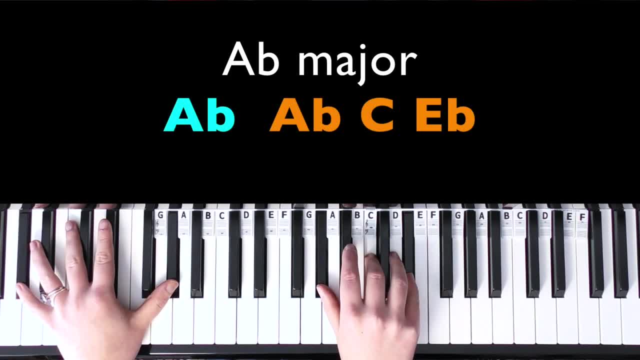 I'm also going to play A flat major, So I'm trying to make this a slightly more interesting chord progression. So it's A flat and then A flat C and E flat, And then we have B flat major. So that's B. 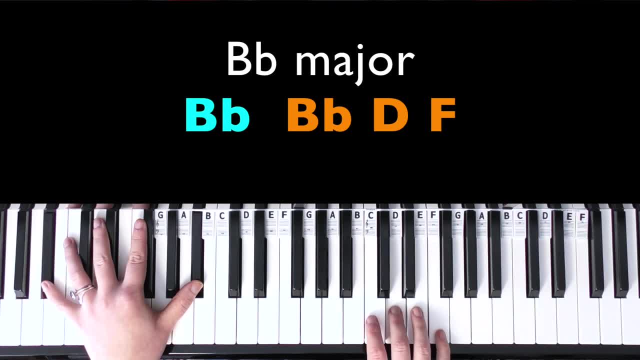 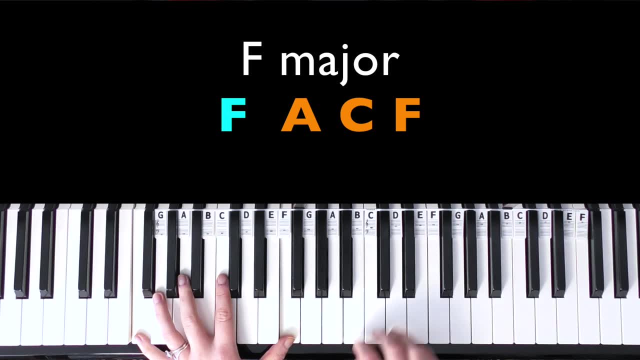 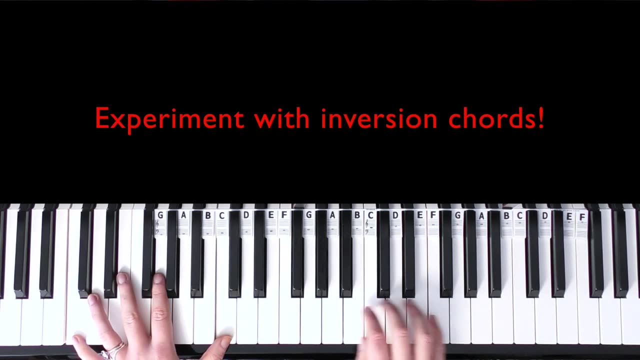 flat, and then B flat, D and F And then F major. I'll probably play it as an inversion, So it's F's and then A, C, F or C, F, And again, you should be experimenting with inversions anyway. 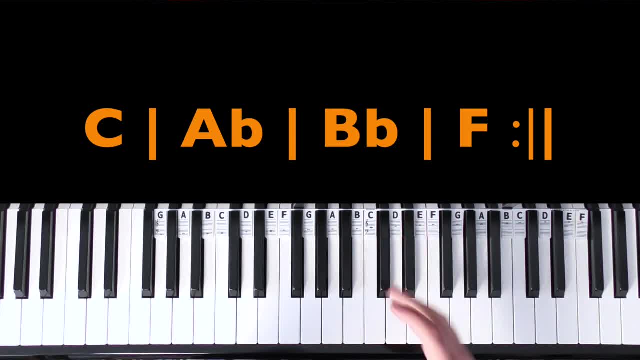 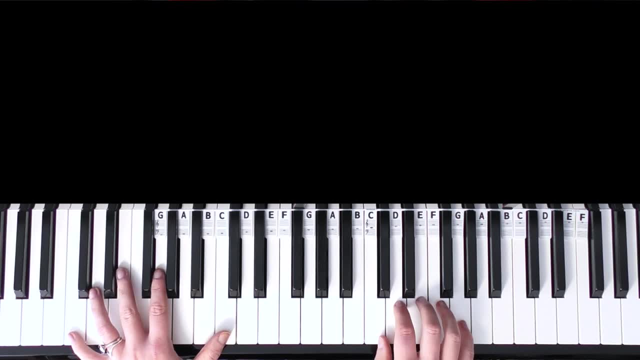 They're the four chords I'm going to be using, So not using any specific songs. So the first one is on the beat with extra thumbs, So instead of playing it just like this, so it's four beats in a bar: 2, 3, 4, 1. 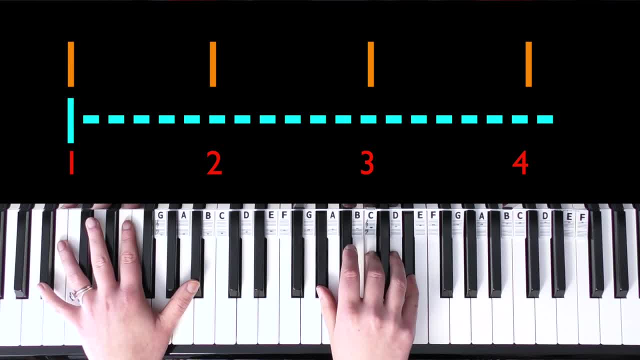 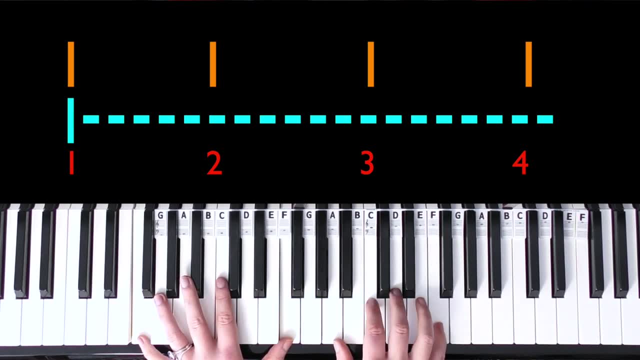 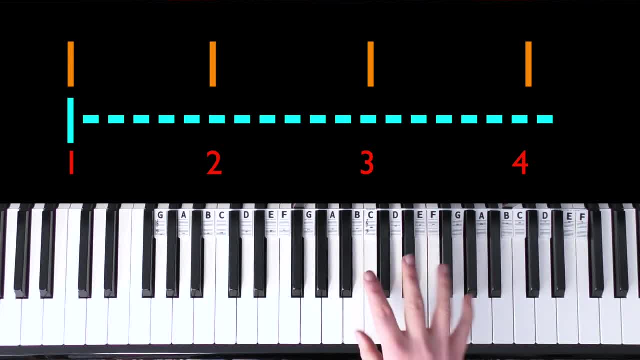 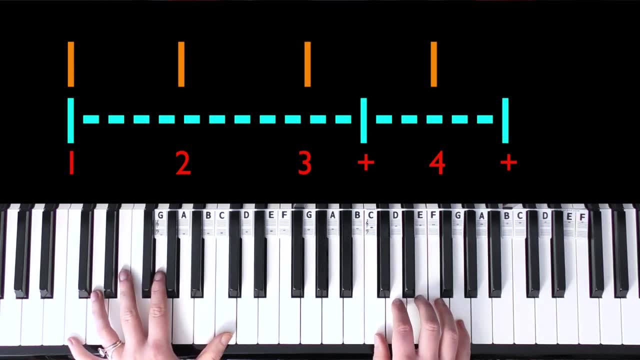 So where you're holding down the left hand and then you're just pulsing, keeping the tempo really in your right hand. So what we could try instead- so this is quite simple- is that, but we're going to repeat the bass note a few extra times. 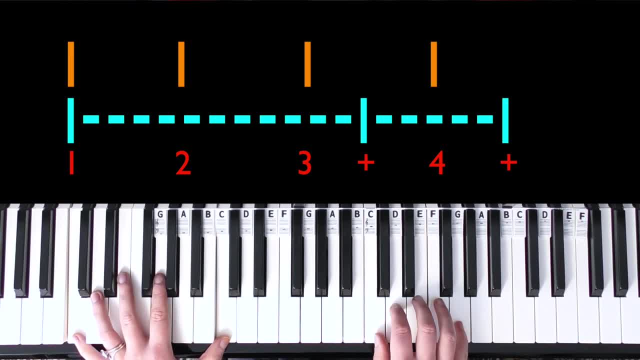 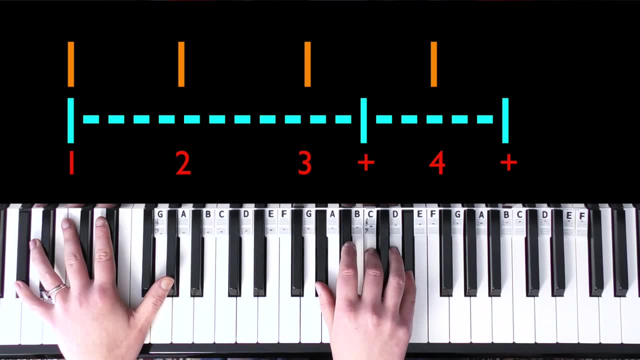 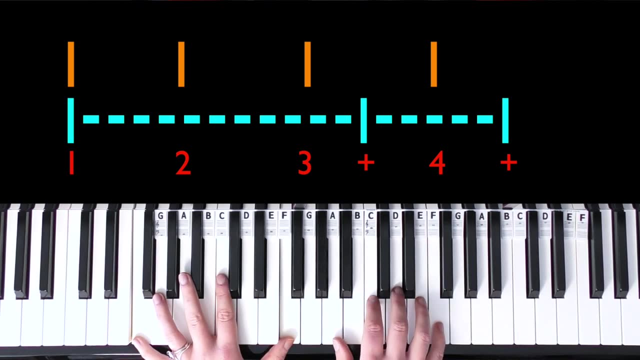 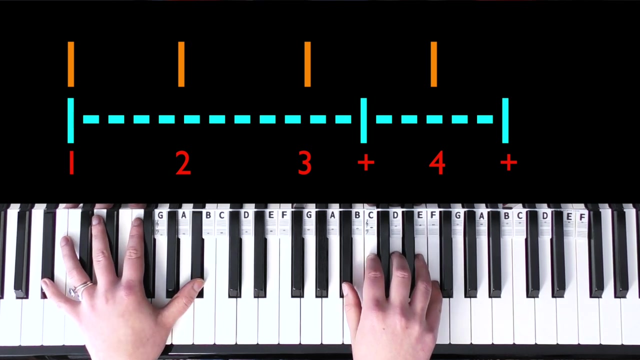 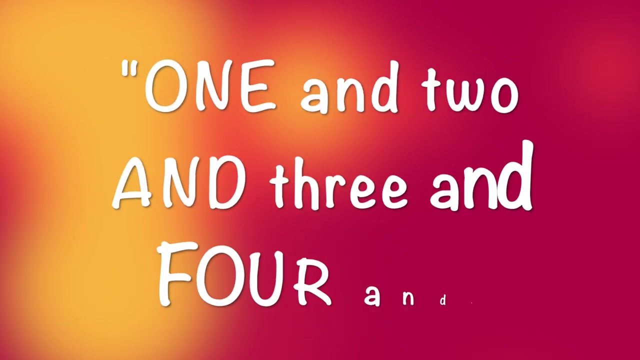 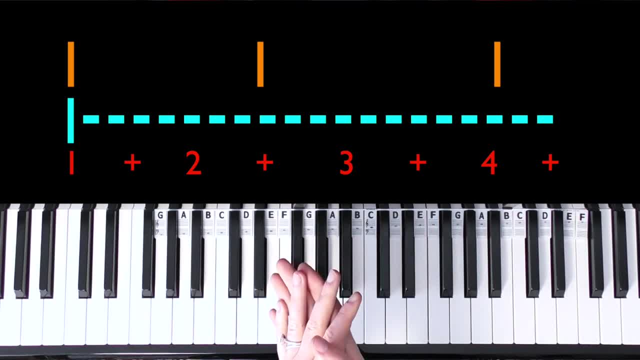 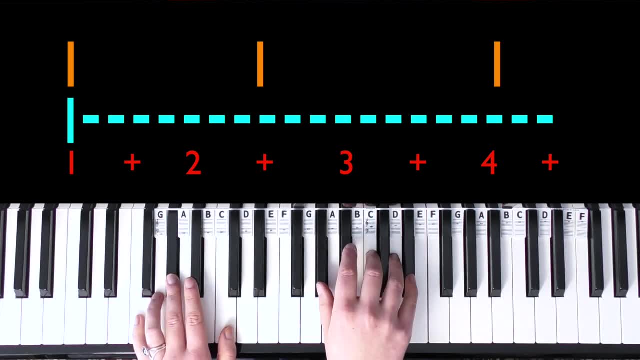 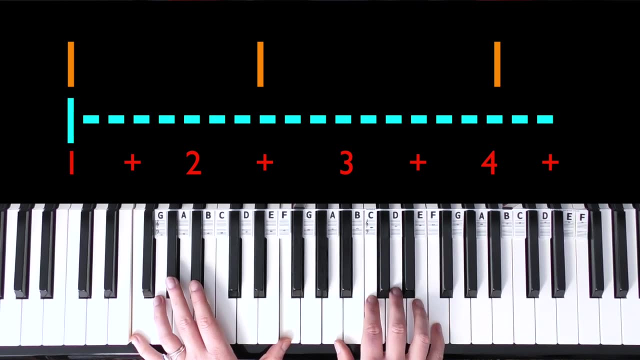 So it's going one and two and three and four and One and two and three and four and four and two and three and four, and So that's a super, super common one where you're playing a little bit of an offbeat rhythm. 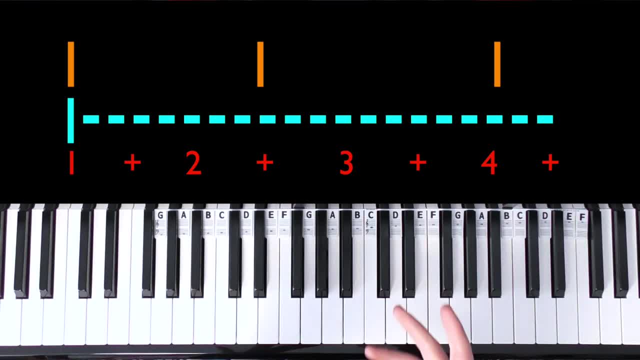 but it's still quite regular to help keep someone in time, So you can incorporate that rhythm and some of the extra left hand notes in between the chords, So something like this: So one and two and three and four, and one, two, three and four and. 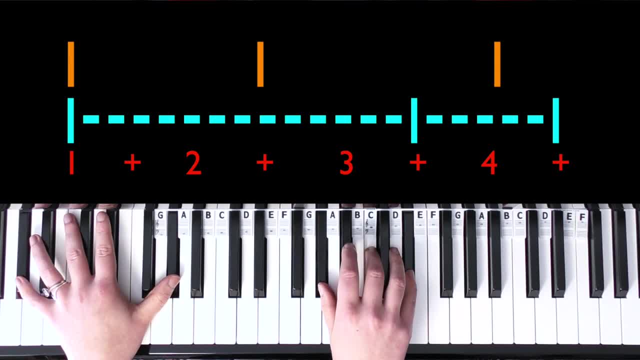 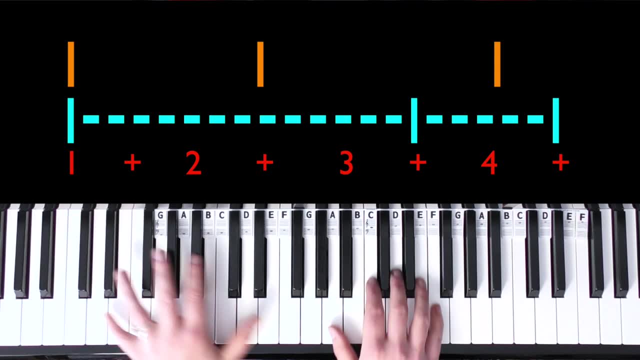 So that's a super, super common one where you're playing a little bit of an offbeat rhythm, but it's still quite regular to help keep someone in time, So something like this: So one and two and three and four and one, two, three and four and one, two and four. 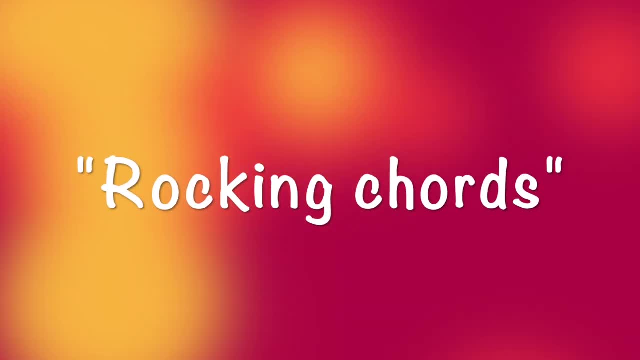 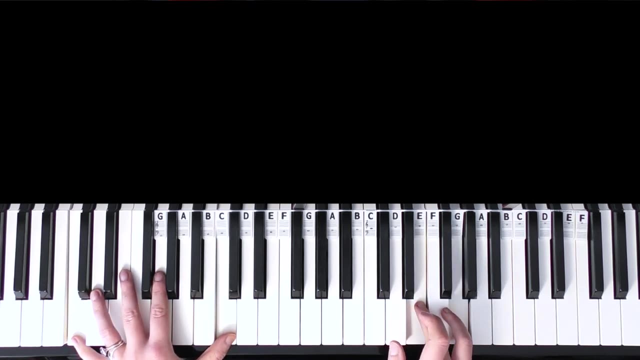 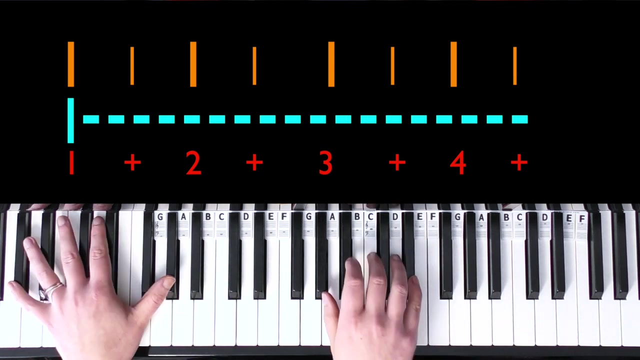 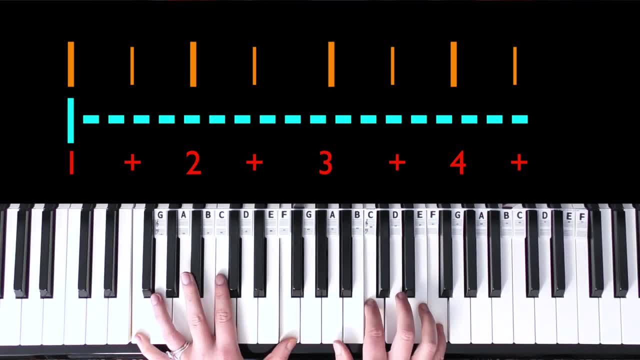 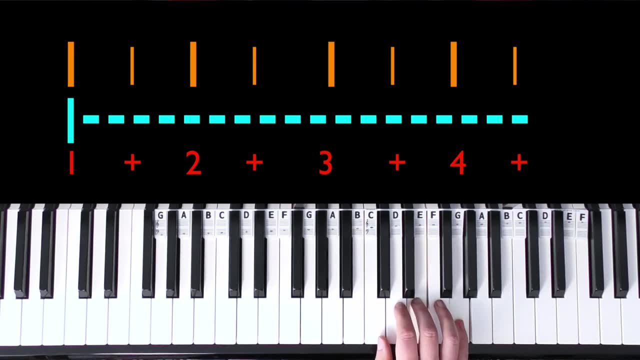 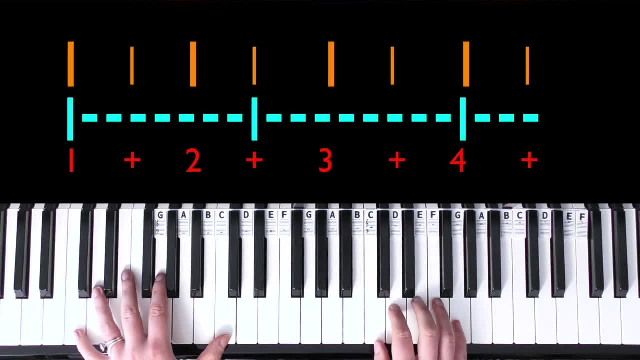 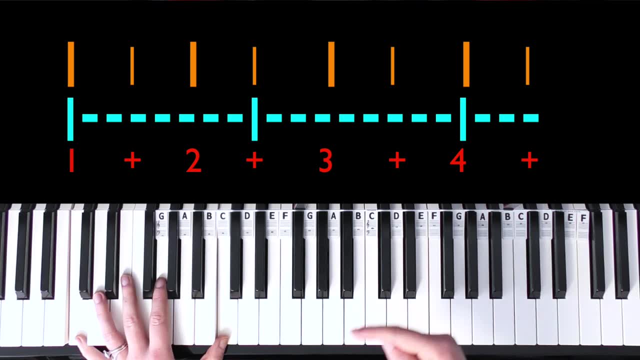 You could again try to incorporate some extra left hand notes, So going one and two and three and four, and So incorporating the rhythm, the accented beats that we had in the second pattern with the left hand, So one and two and three and four, and 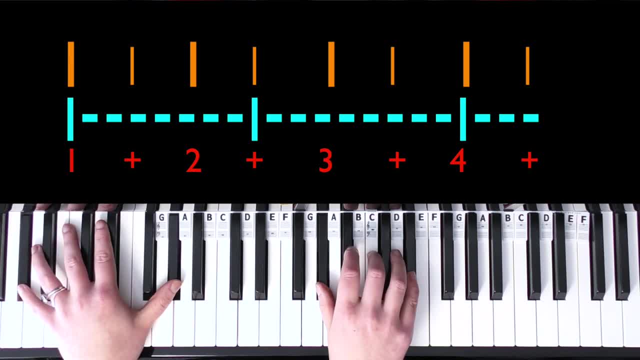 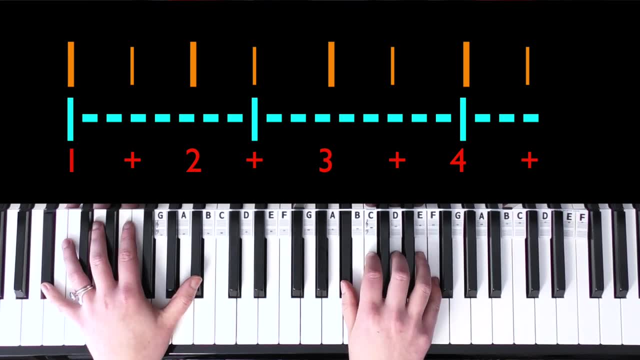 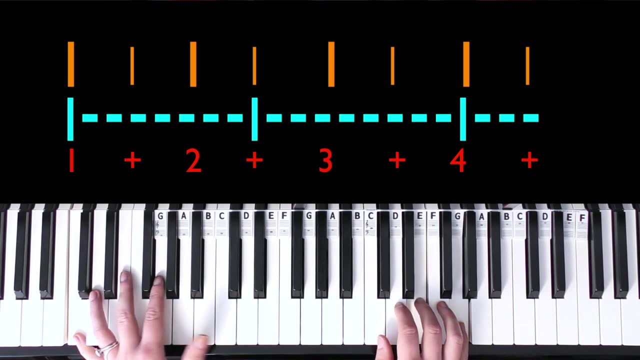 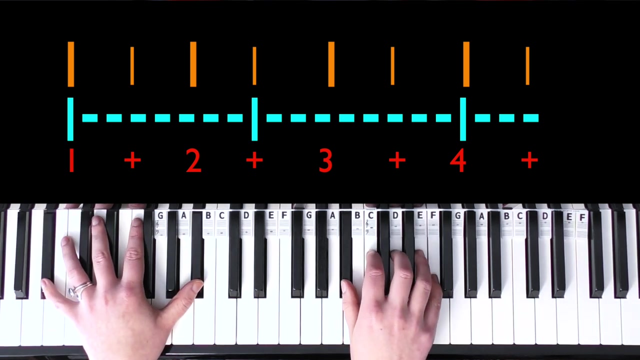 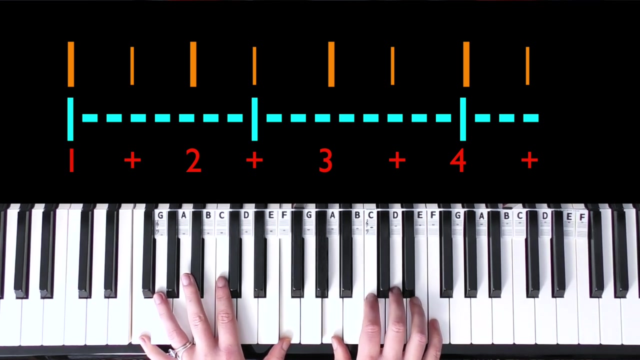 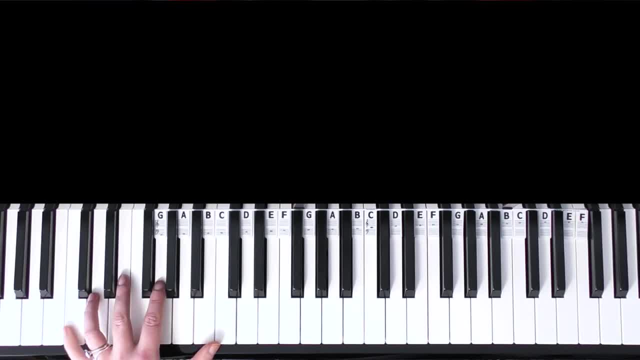 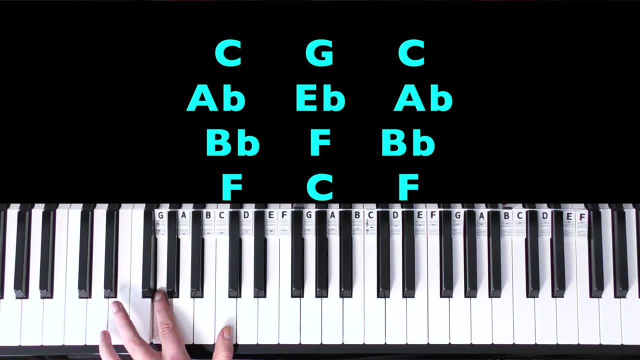 So you don't have to be able to play the octave at the same time, But you have to be able to move from the C, the G and then the next C, like this: So those, Or you can go One and two, and three and four. 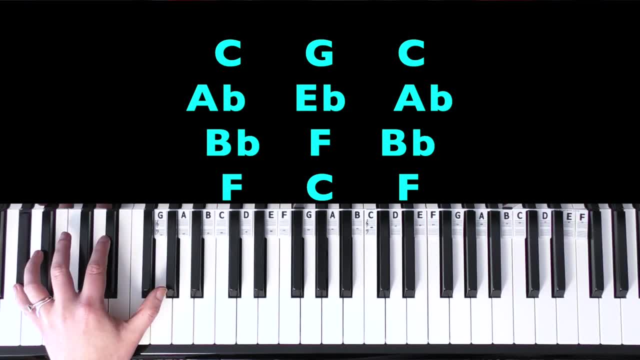 And then A flat, E flat, A flat One, two and three and four and B flat, F, B flat, And then C and then F, C, F, So incorporating the fifth in there as well as the octave, And in the right hand you can just hold down the chords. 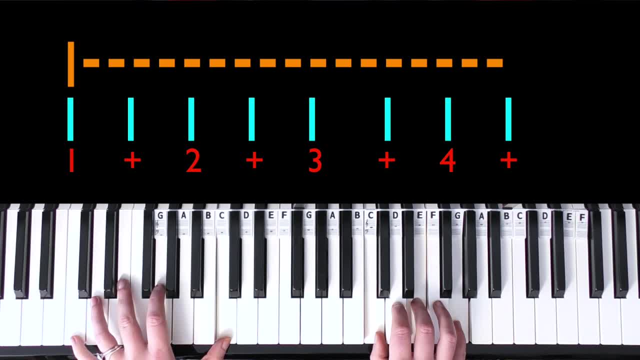 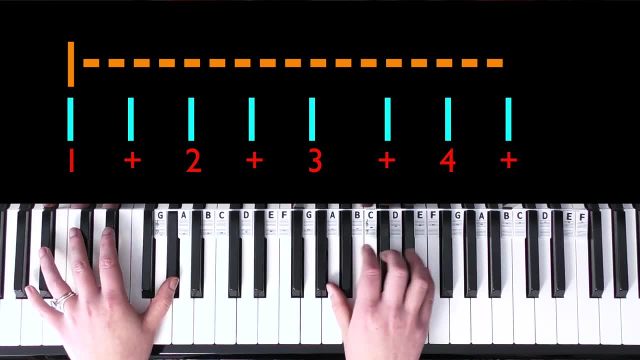 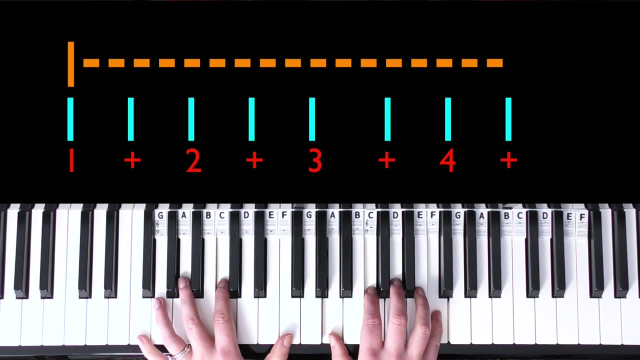 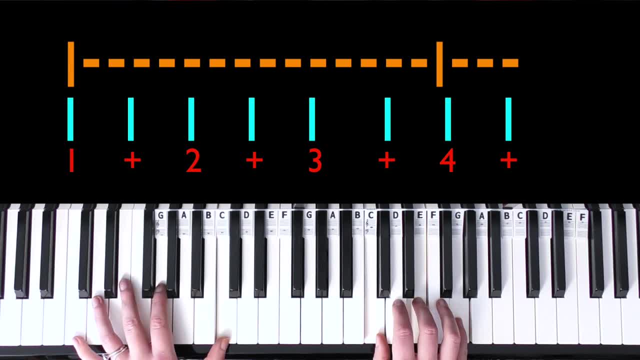 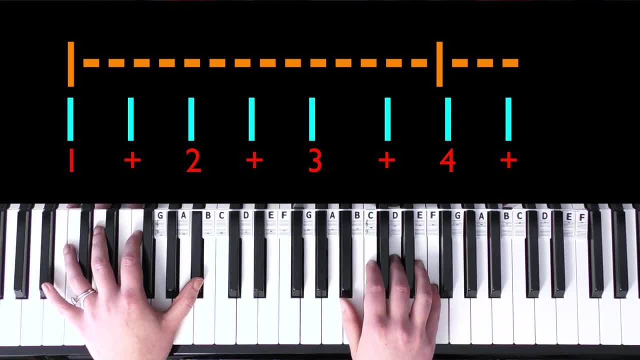 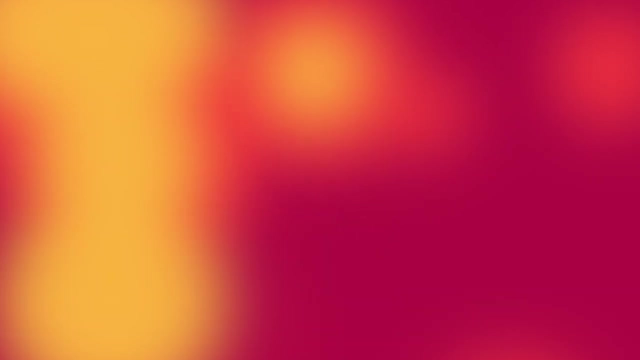 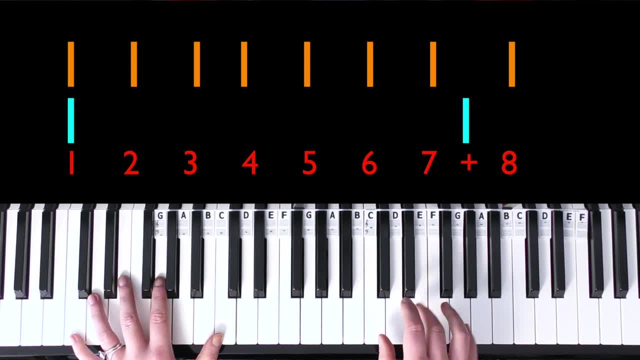 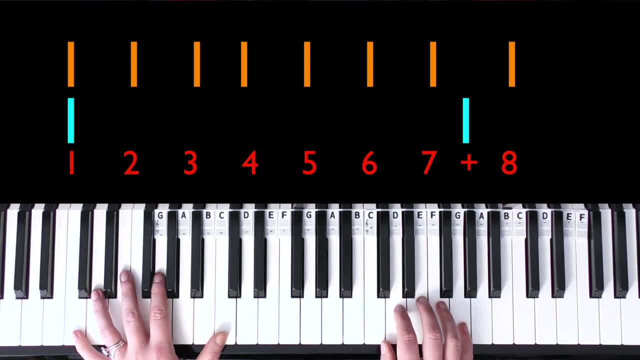 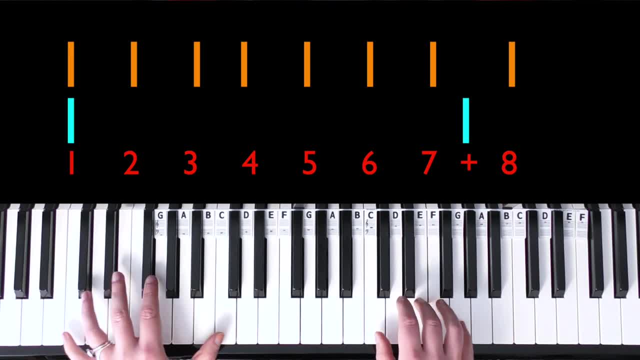 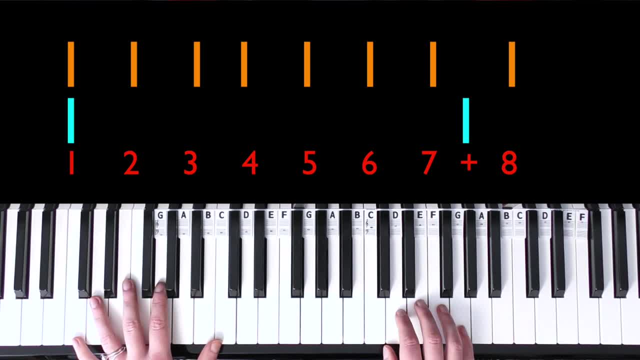 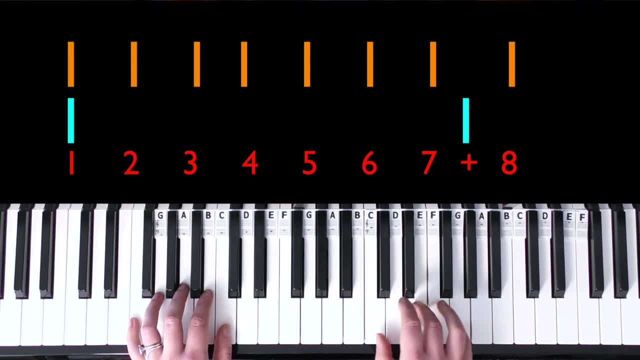 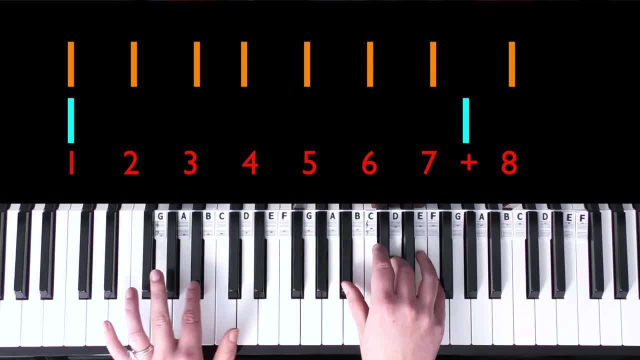 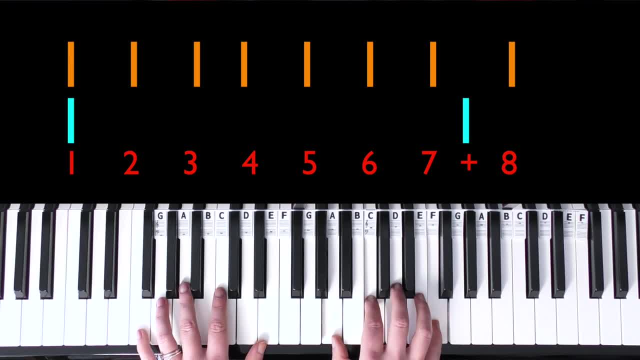 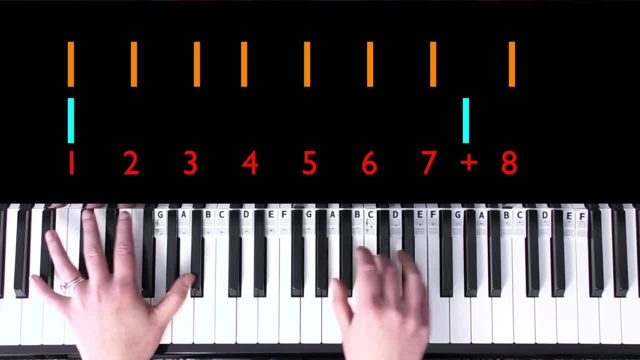 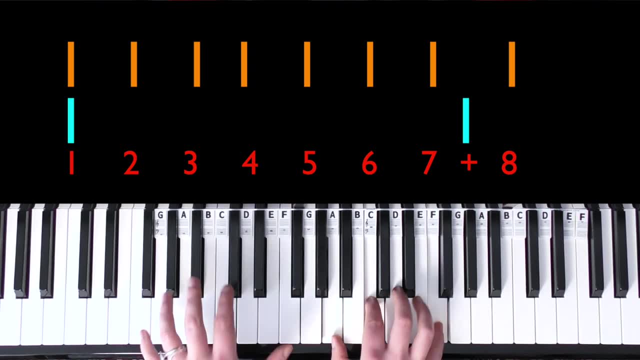 1,, 2,, 3,, 4,, 5,, 6,, 7, 8. 1,, 2,, 3,, 4,, 5,, 6,, 7, 8. 1,, 2,, 3,, 4,, 5,, 6,, 7, 8. 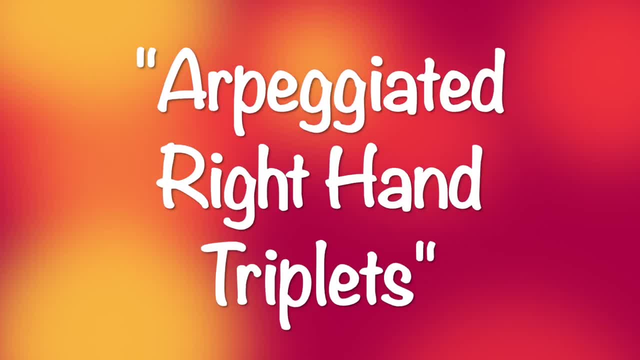 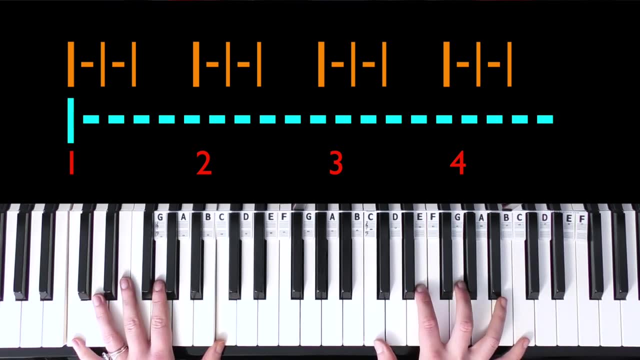 And then the sixth one is arpeggiating the right hand, So in triplets. So we have C, E, G, and then we're going to add the octave of the C on top, Whilst holding the left hand root note of C down. 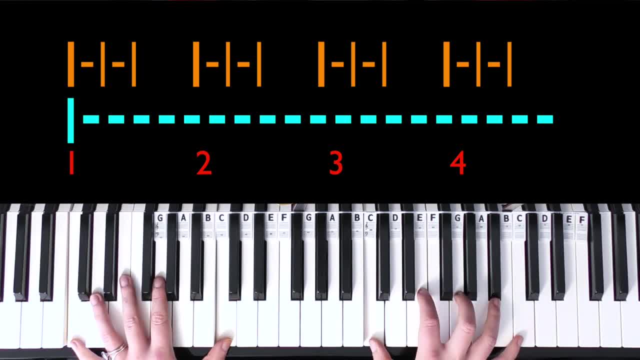 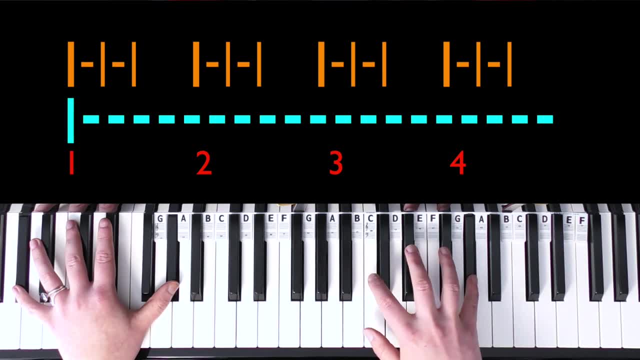 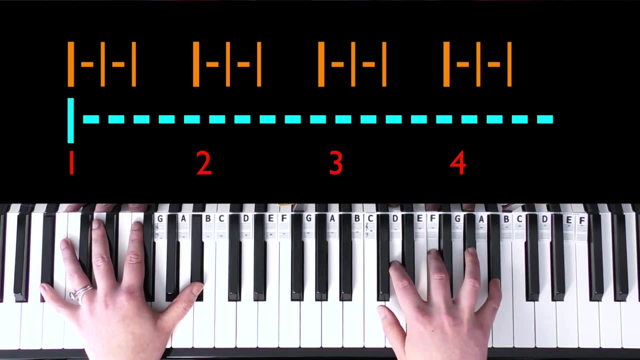 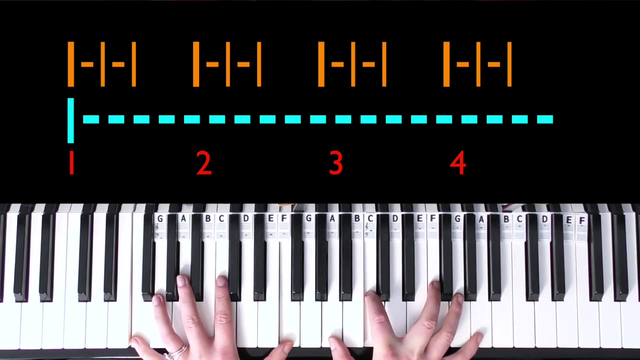 So 1,, 2,, 3,, 4 And then Ab, so Ab, C, Eb, Ab, And then Bb, D, F, Bb, And then A, C, F, A, Complete an inversion. So again, with this one you could add an extra left hand note. 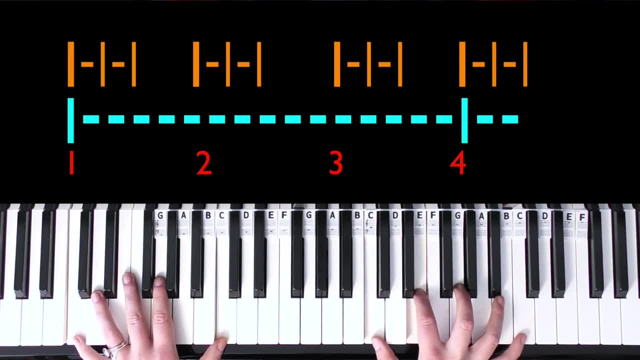 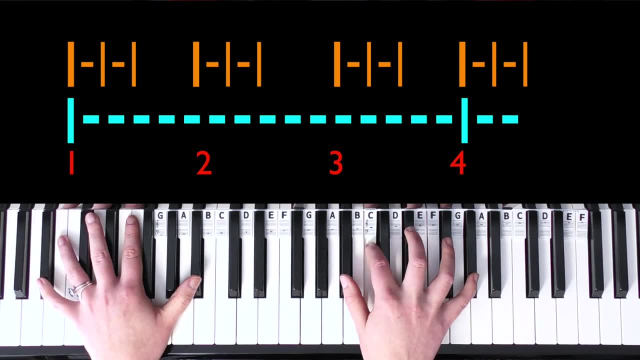 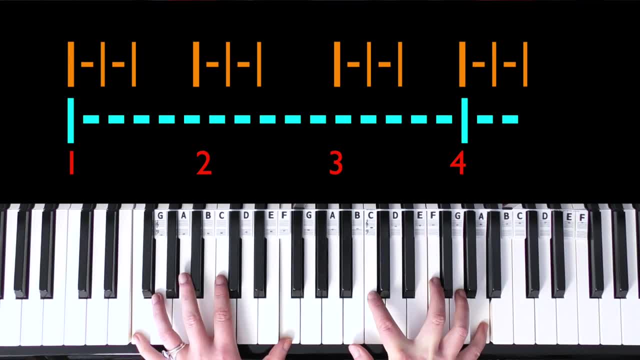 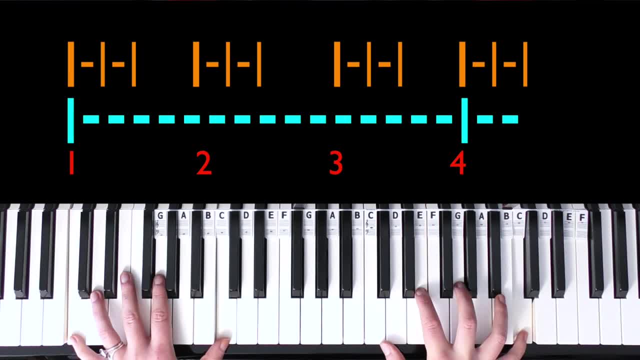 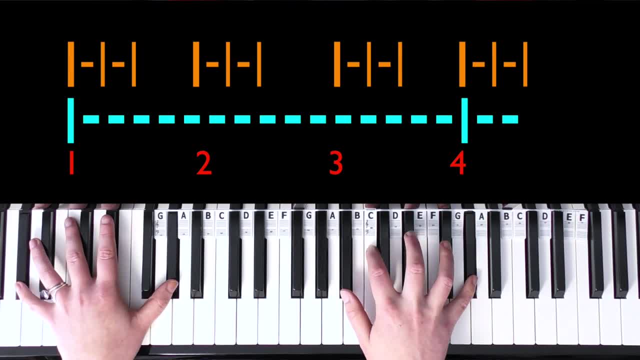 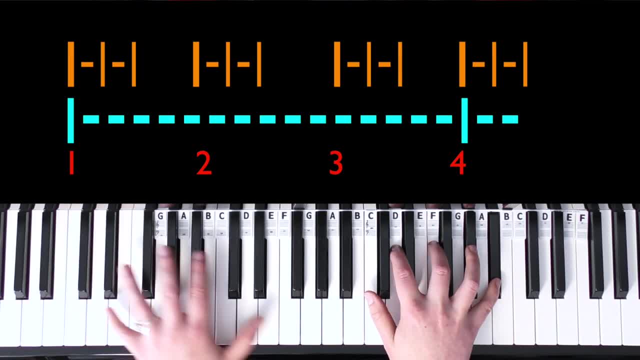 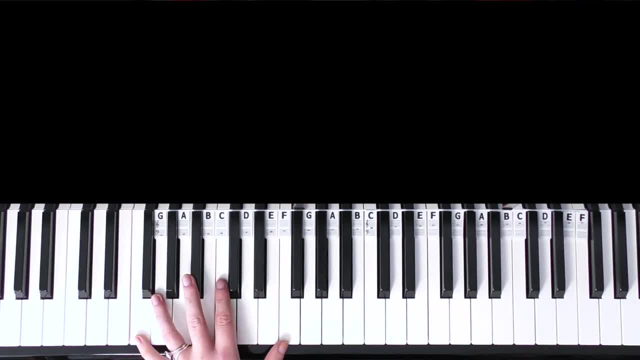 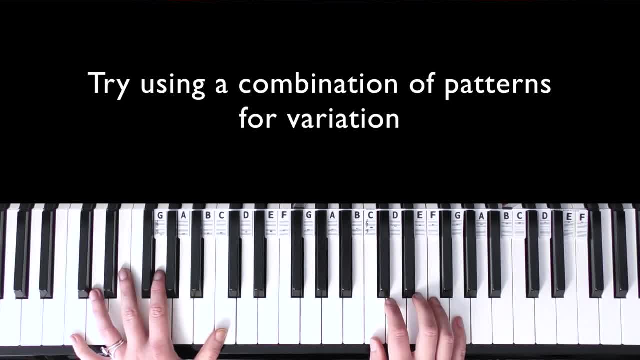 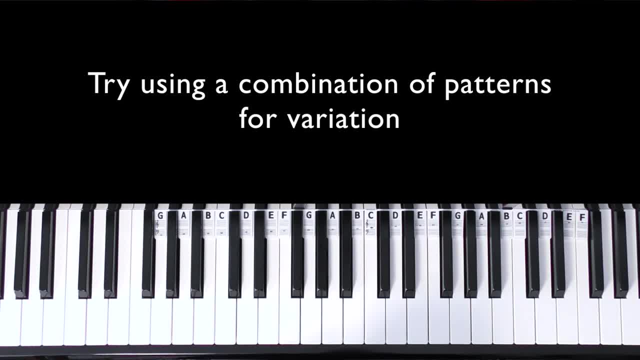 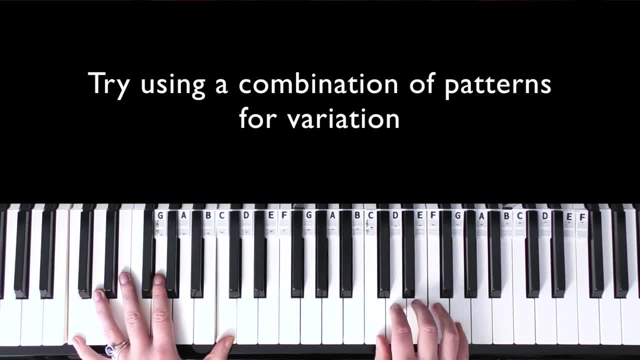 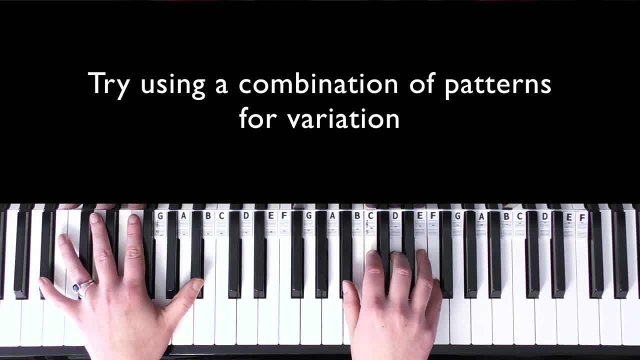 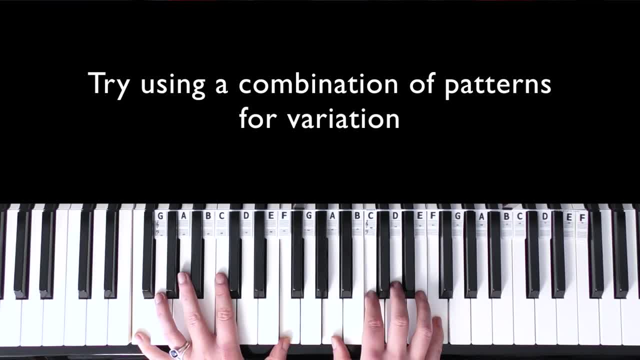 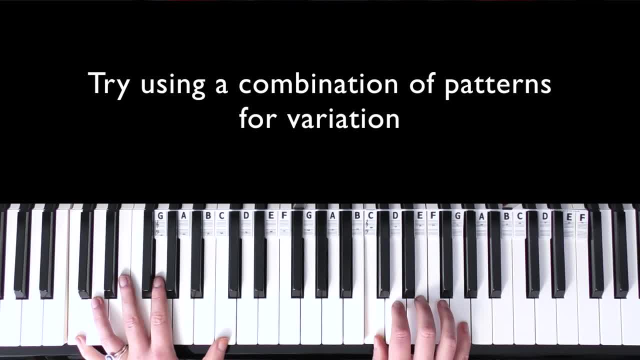 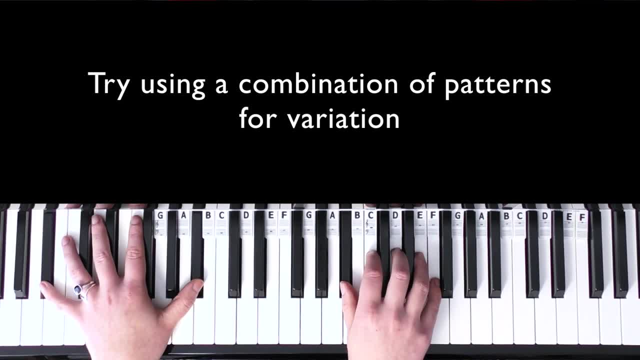 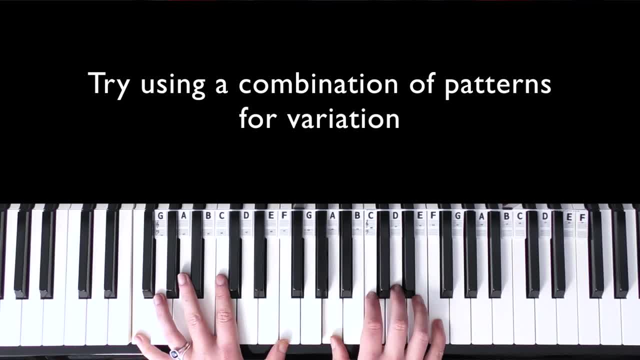 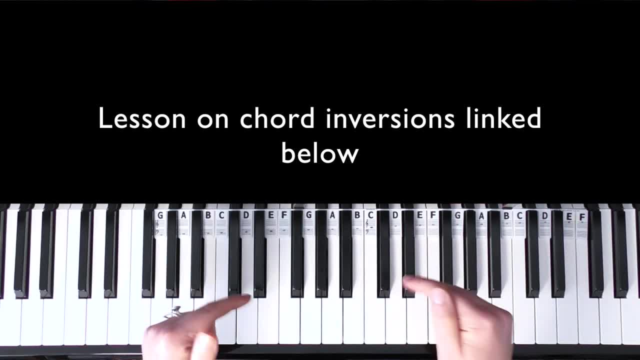 root position chords. of course, If you don't know what the inversions are, you really, really really need to know them. So I have left the video links below. that tells you exactly what they are, why they're useful, how to do them. So I hope you found that useful and that it's 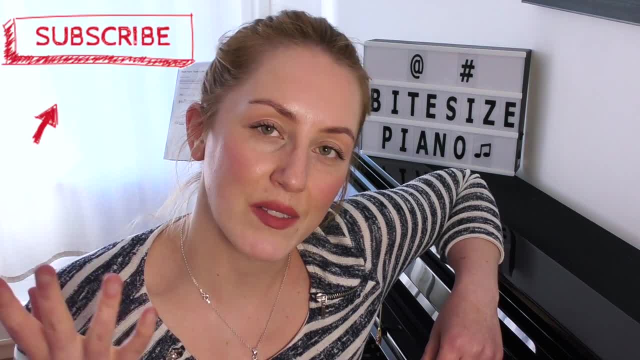 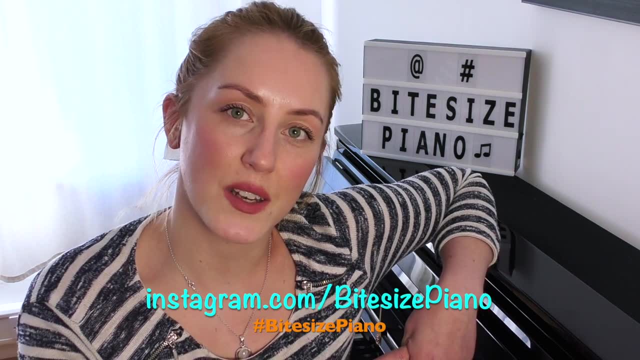 given you a few ideas. Please remember to subscribe, if you haven't already. I would love to have you here learning from my tutorials. Go follow me on Instagram, which is at Bytesayspiano. I look forward to seeing you all over there, and 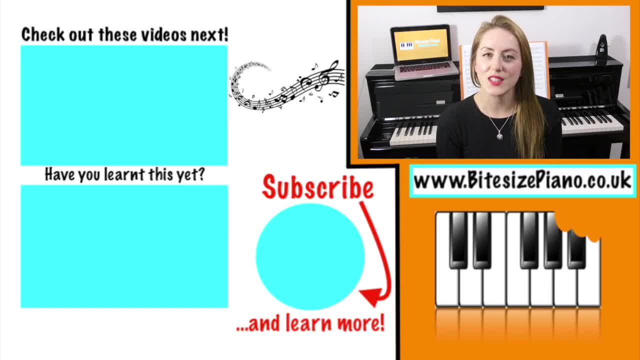 in the next video. So that's the end of this video. If you would like to leave a request, leave them in the comments section below of this video. I've also left some videos here that I think you might like, so go and check those out, as. 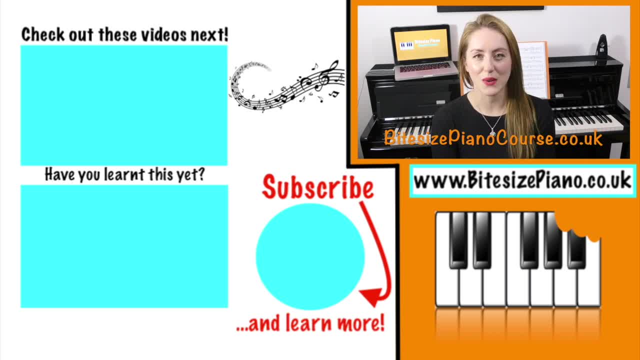 well, I also have a course visit bytesayspianocouk and you can enrol and start learning how to read music. I'll see you in the next video. 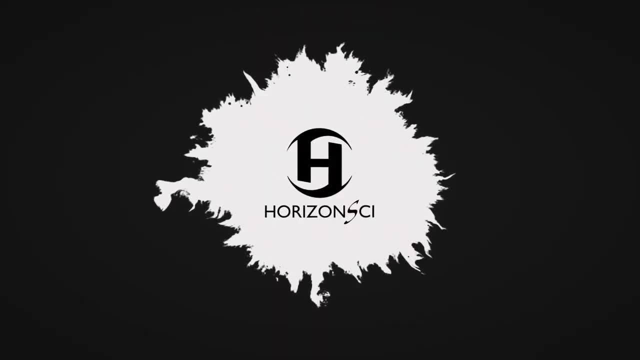 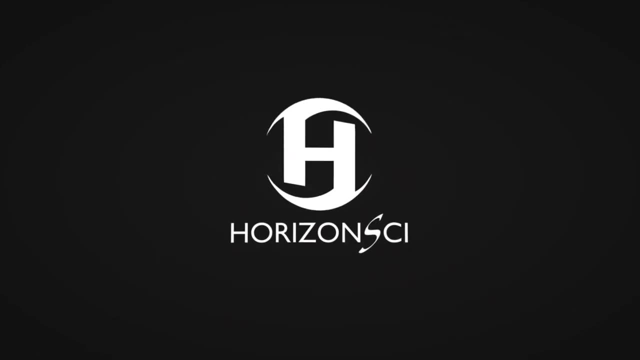 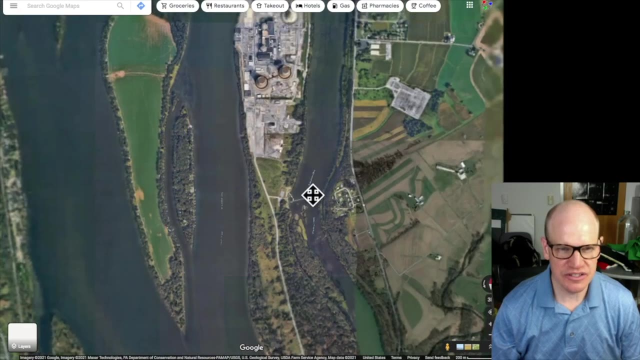 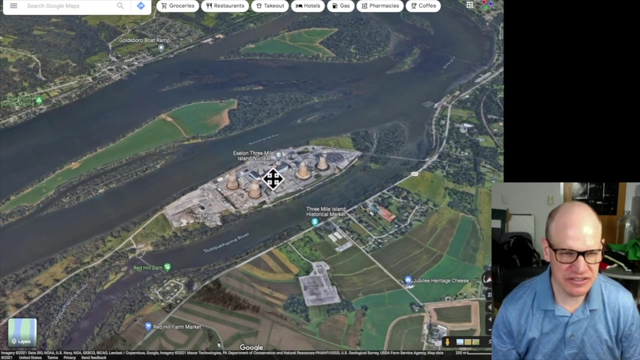 So today we're going to be talking about the design of nuclear reactors and get into a couple of the existing styles of nuclear reactors. This is Three Mile Island, right here. It's even a three-dimensional image of it. How amazing is that? So there are two reactors on this island? Actually, there's only one now that's operating.